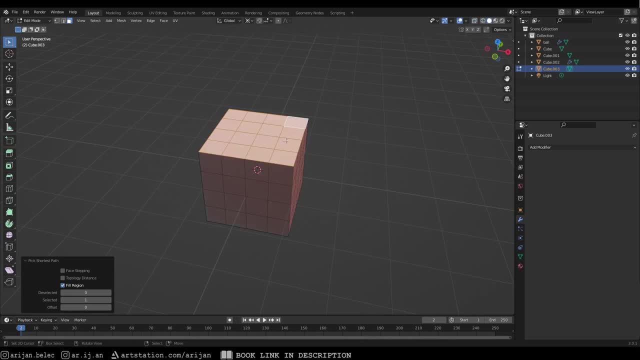 and right click, It's going to select everything between those two faces And then what we can do is just inset the face by pressing the eye shortcut and, as you can see, that's going to start pushing these faces inwards a little bit. Now make sure. 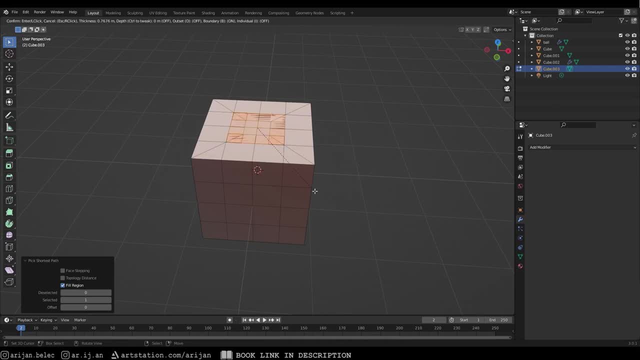 you don't go too far, because then you're going to start getting some of this clipping and overlapping here. So we're going to go ahead and select this entire surface and then we're going to select here. We don't want that, We just want to go somewhere approximately halfway through the. 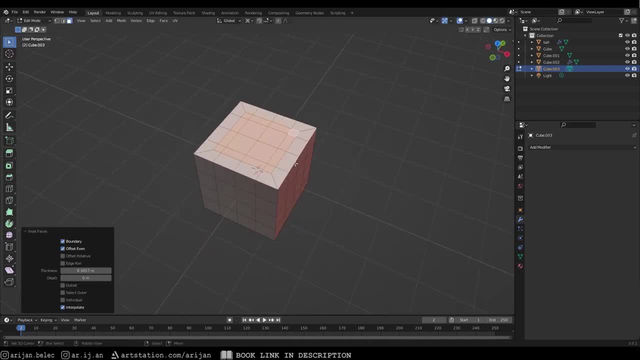 first face or something like this right, And now we can just go to our top view or something. We don't even have to go to top view, but we have to make sure that we have our loop tools add-on enabled for this right. So we're going to go up here to edit preferences and in this little 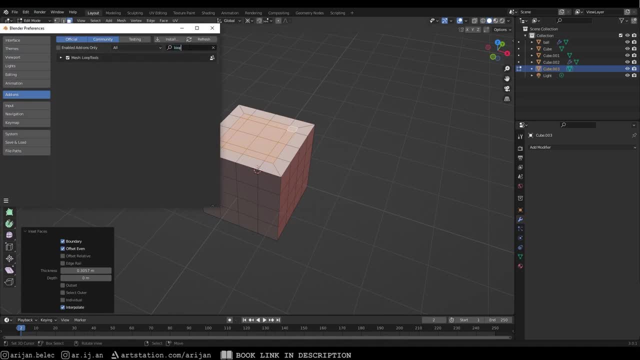 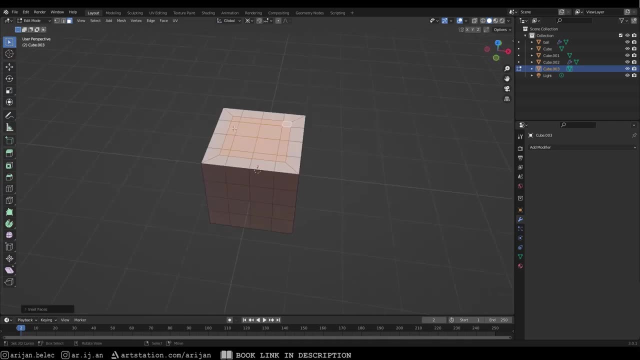 add-ons menu. we're going to search for loop tools. all right, You want to make sure that this here is enabled? all right, It's going to give us a lot of useful tools that we're going to need here today. So once we have this stuff selected over here, we have a loop tools activated. We're going to press. 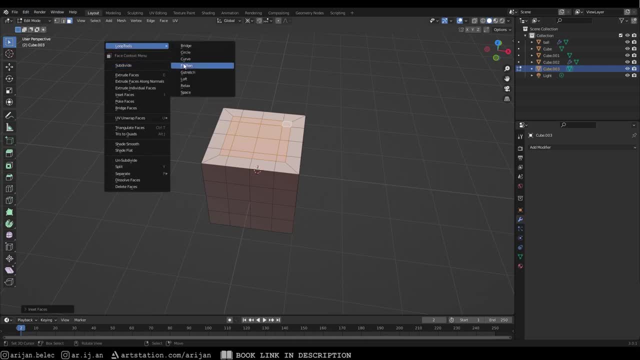 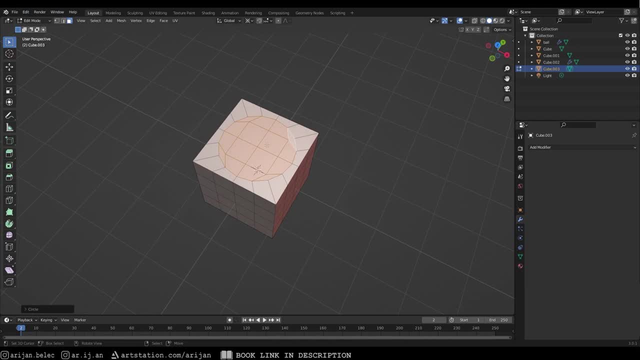 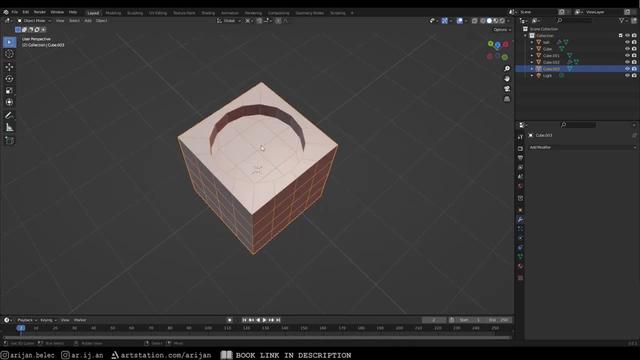 all the faces that we have selected into a circle right. So now this is what we learned in the previous topology tutorial, because now we can just extrude this inwards and we have a perfect circular hole in this object. over here We don't have any weird endgones or anything like that. 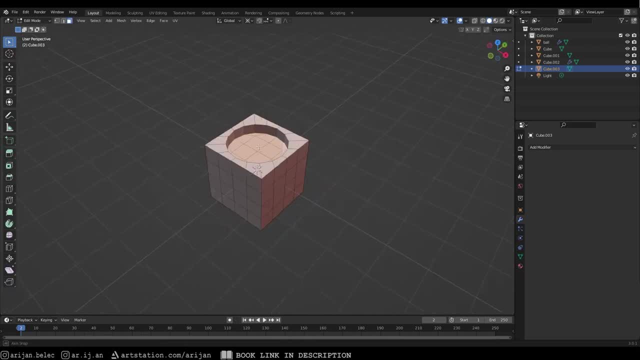 so this is the right way to make a circular hole in an object, right, But we're going to make this a step further because we still have to make the handle or the bridge going across here, okay, So what we need to do now is we have to delete these faces on top. 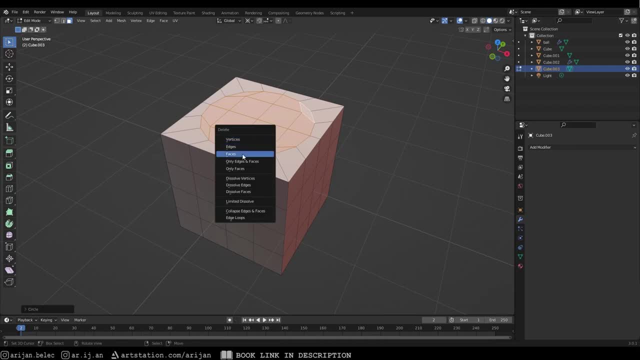 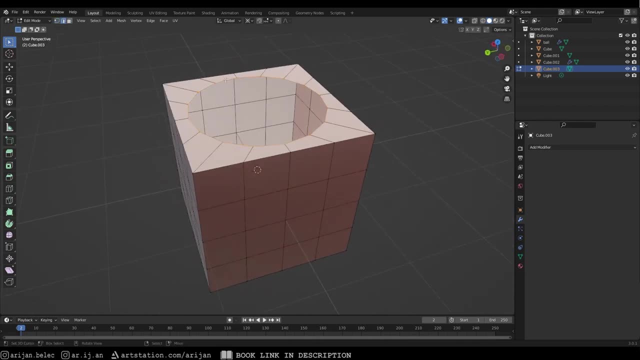 Okay, so we're just going to press X and delete the faces on top here. So now we just have a circular hole, a circular gap here, which we can see inside the cube through all right Now, to make this little bridge that goes over, we're going to have to get started by first. 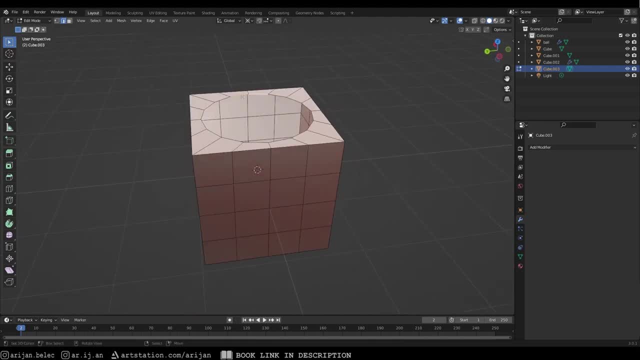 connecting a couple of the edges here. So we're going to select two edges here on one side- or maybe you can select a few more if you have a more detailed circle or something like that- but I'm just going to go with two because that works best for me. here I'm going to select two. 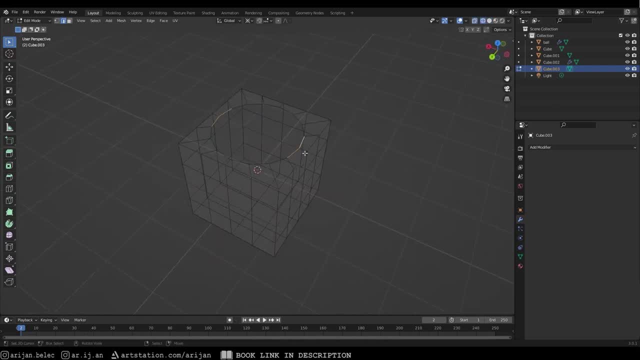 edges on this side and two edges on this side. And now when I'm in edge select mode, which I can access By pressing the 2 button, all right, Or I can also press this over here to select edges, as opposed to vertices or faces and stuff like that- We select these two edges on opposite sides over. 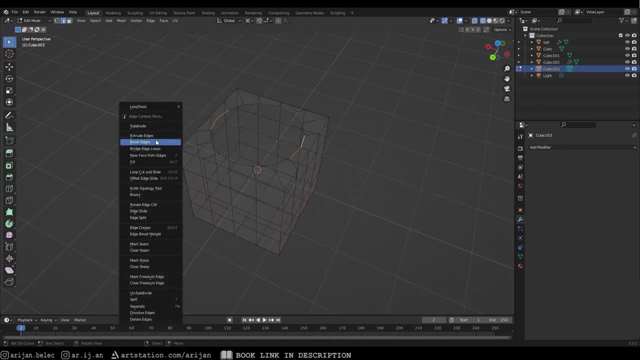 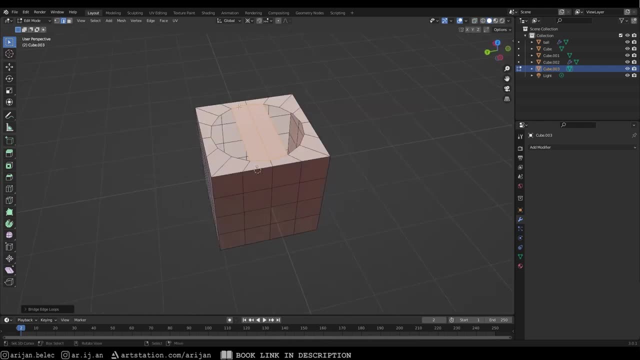 here and we press W and we're going to go over here to Bridge Edge Loops And, as you can see, this also instantly connects these two edges that we have selected on the opposite side of the circle. right Now, we have to make this bridge look a little bit nicer, right? So we're going to 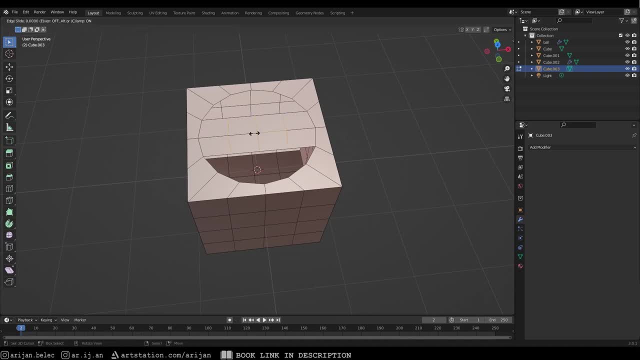 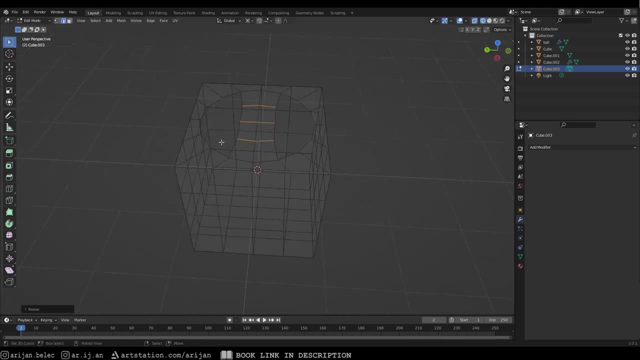 add a couple of loop cuts, let's say three loop cuts, okay, here on this bridge with Control-R, and we're just going to scale them down on the Y-axis A little bit, or whatever axis you're doing this on right, Just to make them a little bit more. 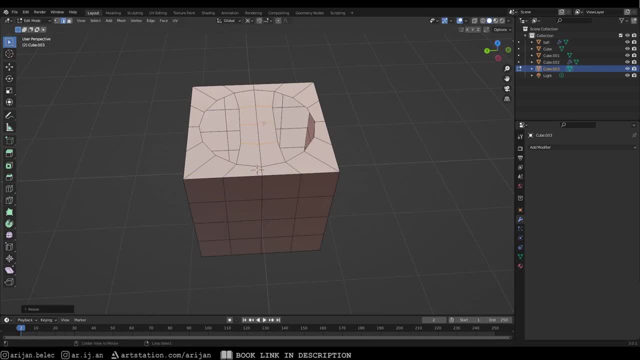 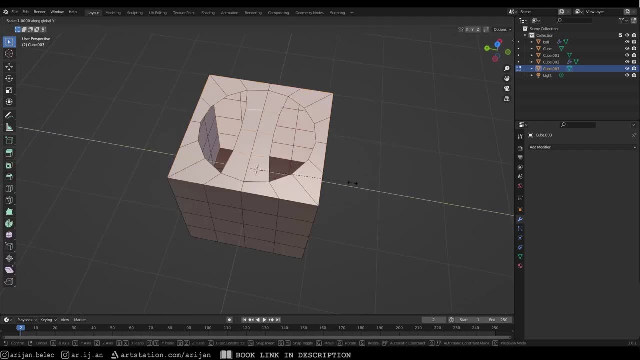 narrow because, as you can see now, this makes it look like it flows a little bit better, It's a little bit smoother, it's a little bit more rounded, instead of just being a blocky bridge. right, You can take it as far as you want, to make them as narrow as you like, just make sure they. 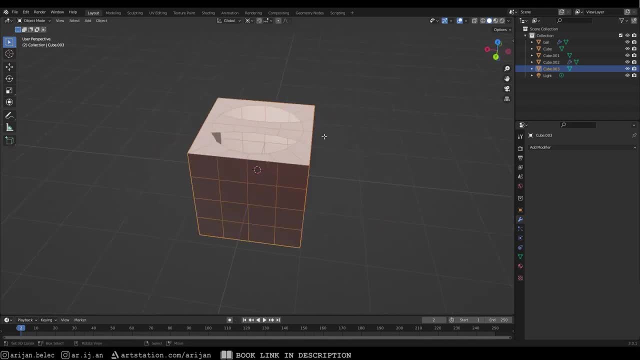 look a little bit smoother right Now. another thing we're going to do to make this look a little bit more round and smooth is we're going to take this edge loop that surrounds the cube over here, okay, with Alt and the right mouse button, and we're going to push this entire edge loop downwards. 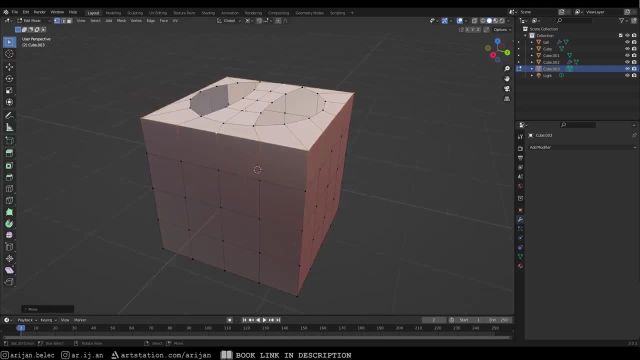 just a little bit Right, So it looks a little bit like it's a little bit inclined or something. so it's a little bit below the circle that we have on top right, And once we do that, we're also going to have to do something similar to the bridge over here. 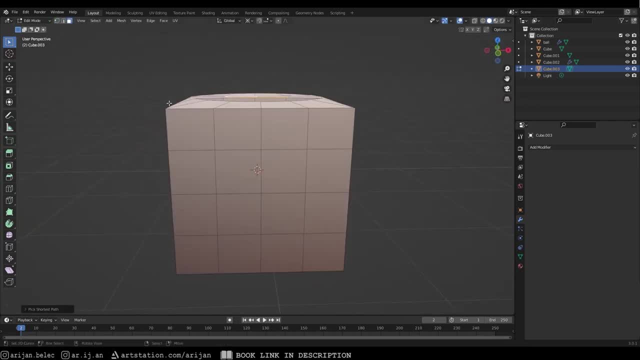 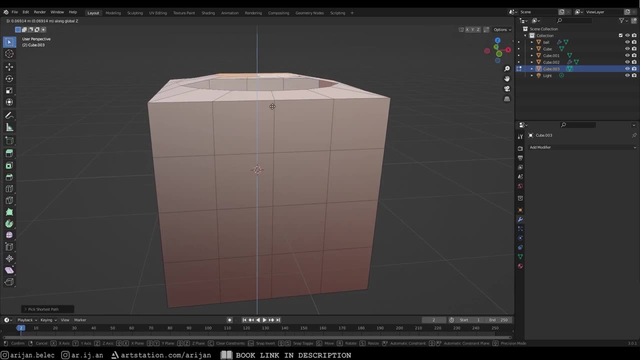 to continue this kind of trend of just kind of arching over the top right. So we're going to select these four faces that we have in the middle and we're going to slightly lift those up, all right. And we're also going to do the same thing once again with the two edges in the middle. 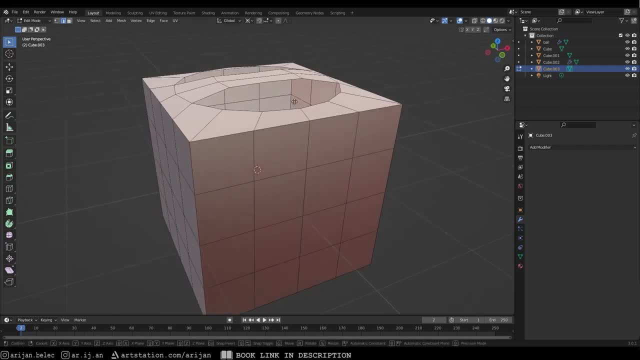 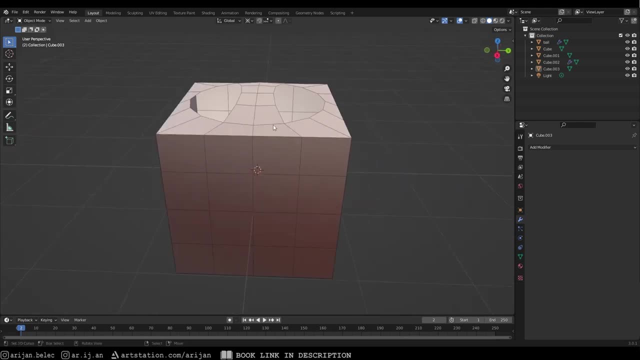 over here in the middle of the bridge. We're also going to lift those up a little bit more, just so we have this round, smooth shape on top. as you can see, now it's all kind of nicely curved and bent on top here. So now we have a good start for our bridge and now we have to start making the 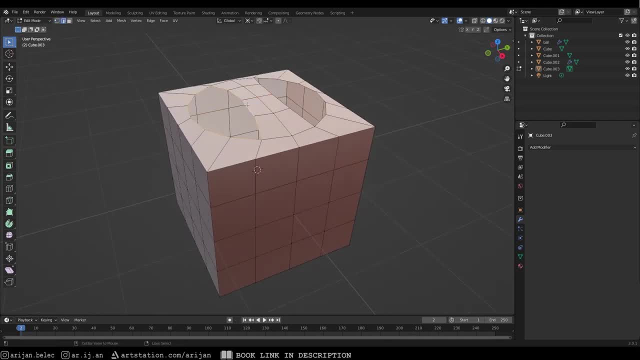 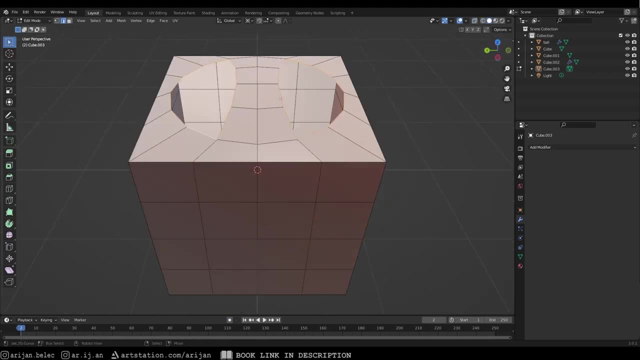 hole below, all right. So what we're going to do now is we're going to select the two edge loops around the two holes that we have. okay, So we have these two holes over here. we can just Alt right click again to select edge loops and we can extrude that. we're going to snap it back into. 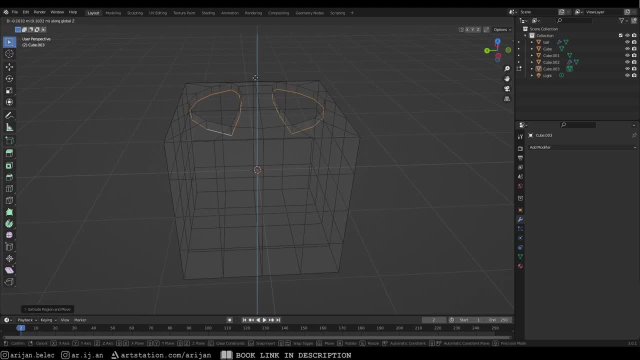 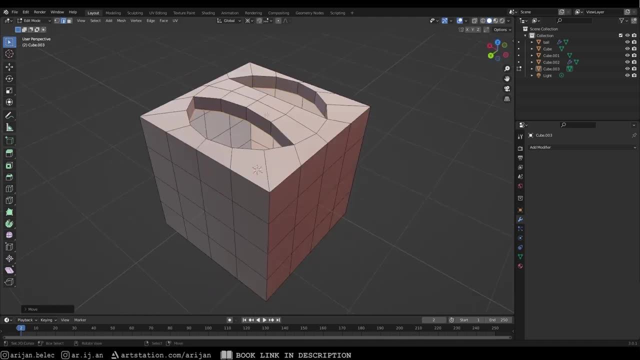 place with right click and then we're going to push that downwards a little bit like this. all right, So now we have this physical bridge forming over here. it has some dimension, has some thickness to it. all right. Now the problem is that we see a lot of people who are 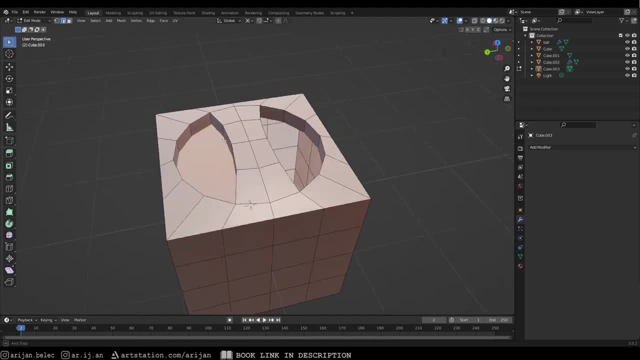 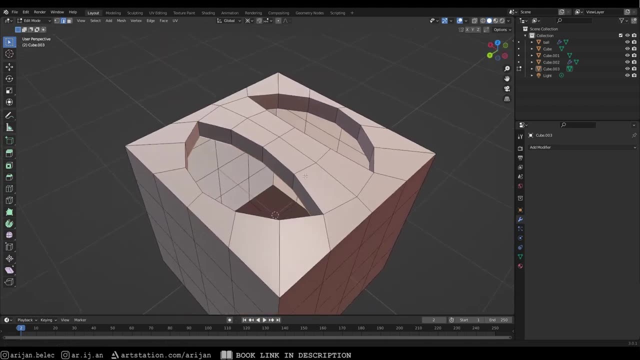 still have the holes at the bottom. we don't want to fill those, because there has to be another gap. this has to go over an empty space now. it can't just be touching the bottom like this right. That's one problem, and the other problem is that if you look below this bridge, it's still an empty. 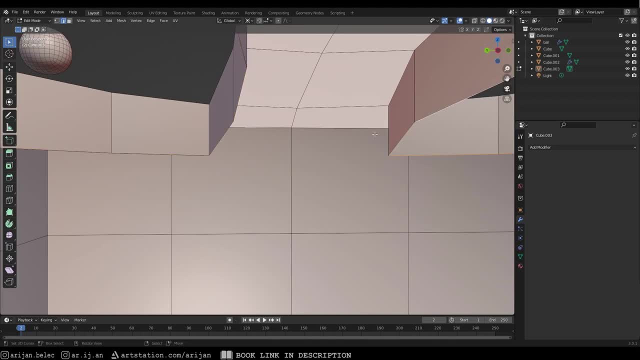 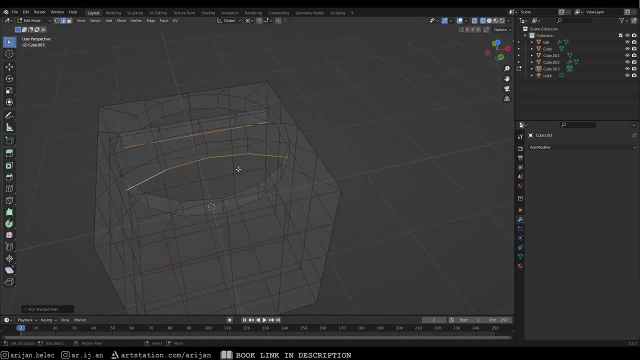 space over here. the faces here are not filled, so we have to fill those in correctly. okay, So we have to select all these edges on the side here at the bottom of the bridge. all right, Let's do that, and once we have those two edges selected, we're going to bridge the edge loops again. 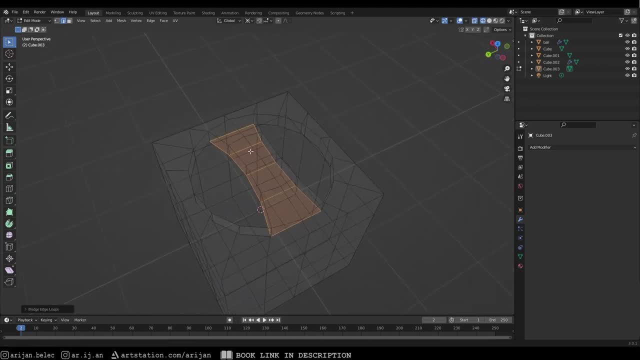 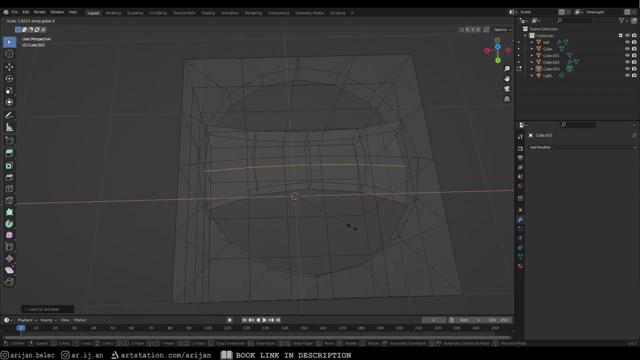 so W bridge edge loops and we're also going to add another loop cut to this to the bottom of this bridge right. So with control R we're going to add a loop cut there. maybe we can make that a little bit longer like this so it kind of fits with the circle above right. We can make. 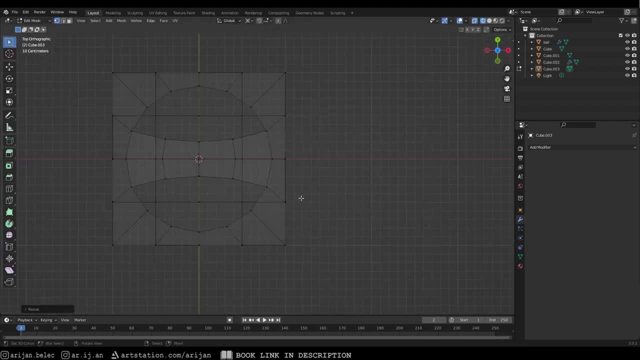 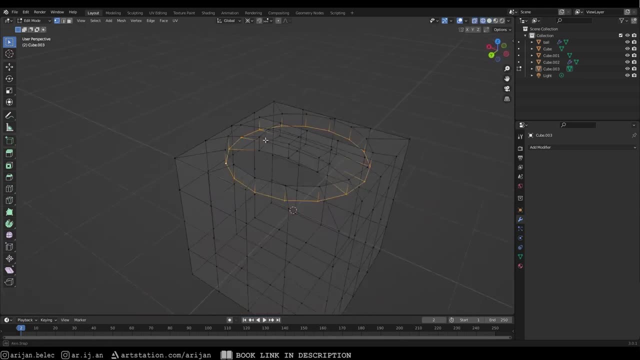 sure, we adjust that a little bit, all right, But now we have these couple of faces connecting the bottom of the bridge. and now we're almost finished, guys, because now we just have to select this edge loop at the bottom once again. it should select all these vertices here, even below. 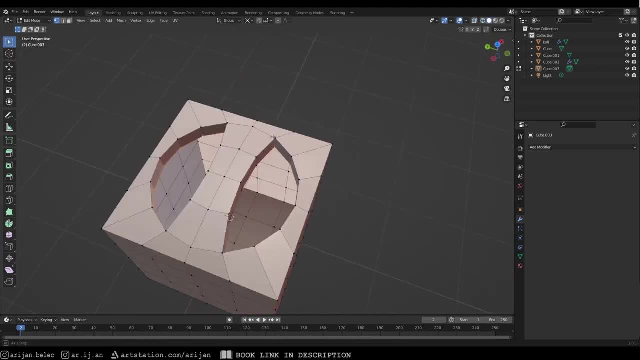 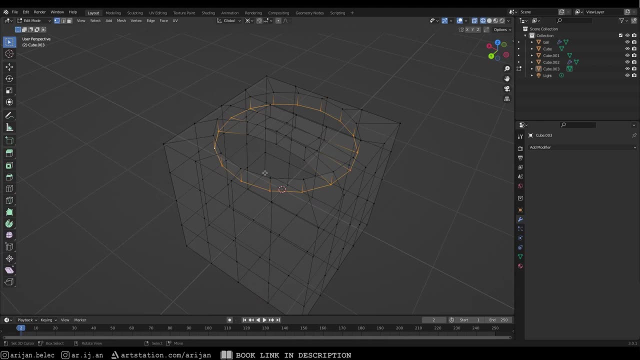 the bridge, which should be in a perfect circle- all right, Or at least close to a perfect circle, because we manually scaled this, so it's not exactly below this vertex, but it's roughly there. and then we're going to extrude this once again with E and we're going to right click to snap. 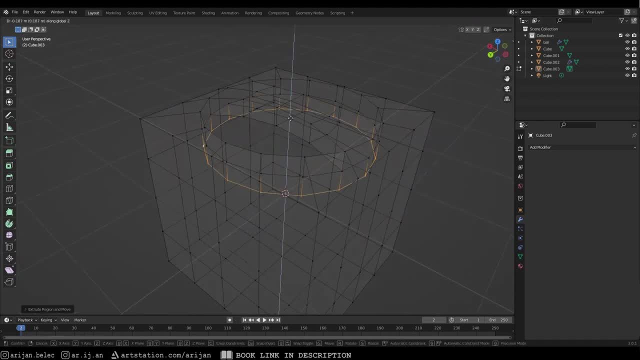 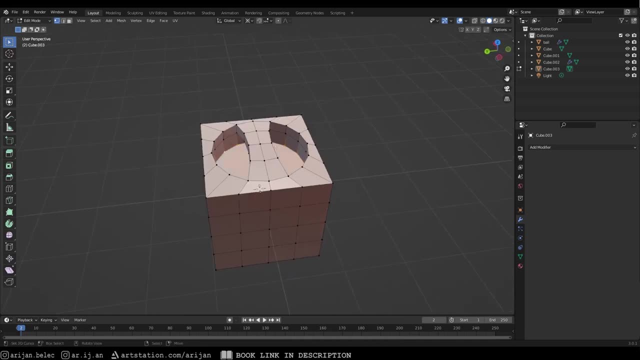 it back into place and we're just going to move it downwards a little bit once again, okay. So now we have this nice space below the bridge. Now we can't just fill this, because that's going to give us a very ugly end. gone, right. So we have to figure out a better way to do that, okay, And 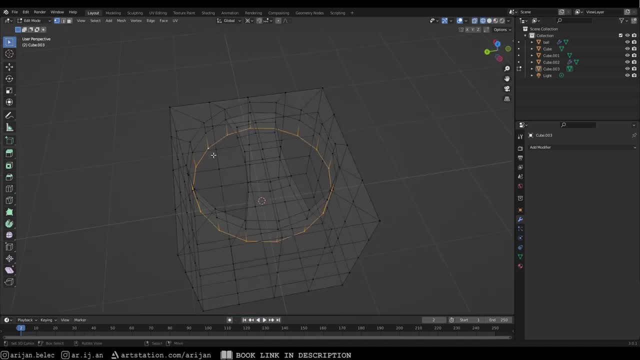 the best way to do that is, while we have this entire edge loop selected, we're going to go up here to the face menu and we're going to select grid fill and, as you can see, this makes a very nice fill. it fills the gap here with a very beautiful looking shape. the topology and the 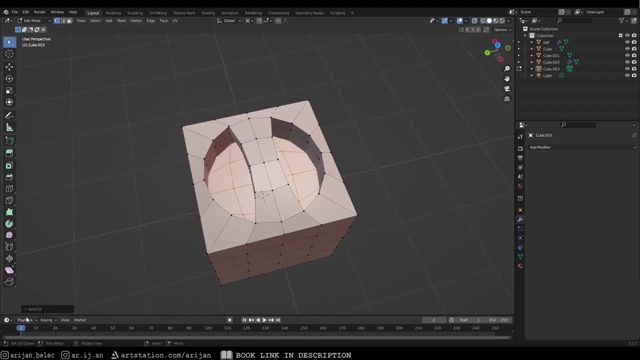 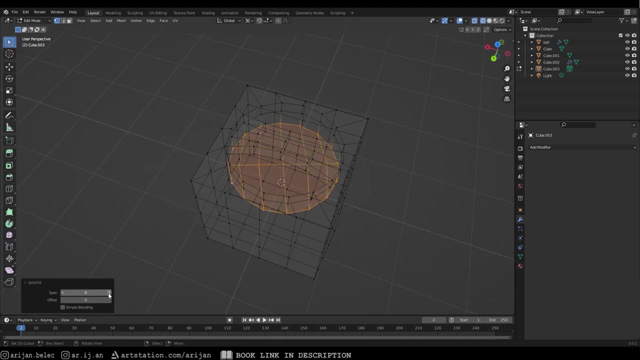 bottom. this is only quads. it's perfect, right? We get this little menu down here. when we use grid fill, we can adjust the way that it fills the shape here. okay, If you look in wireframe mode, you can adjust the way that it fills the shape. if you want to do something a little bit different, 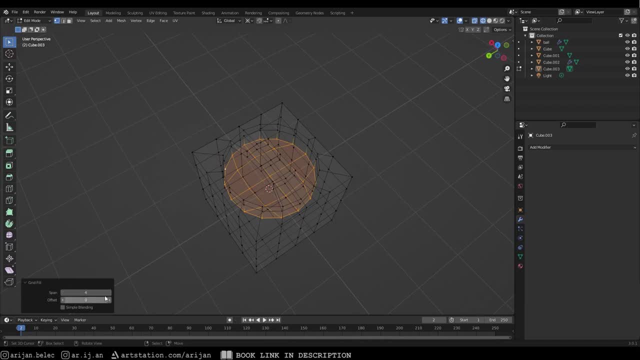 if something is a little bit more suitable for your particular situation, you can tell Blender how to fill this exactly. you can have some control over this right. For me, the default way that happened here right now works perfectly well, so I'm going to keep that. And after we do that, 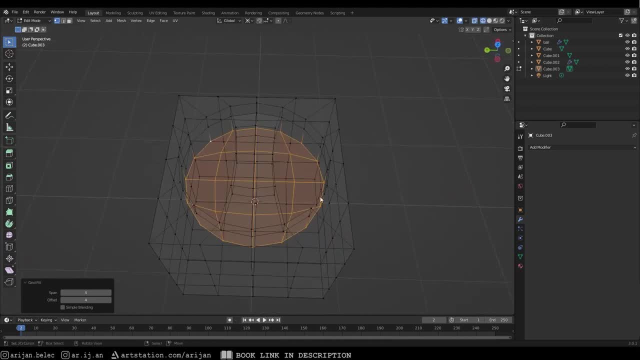 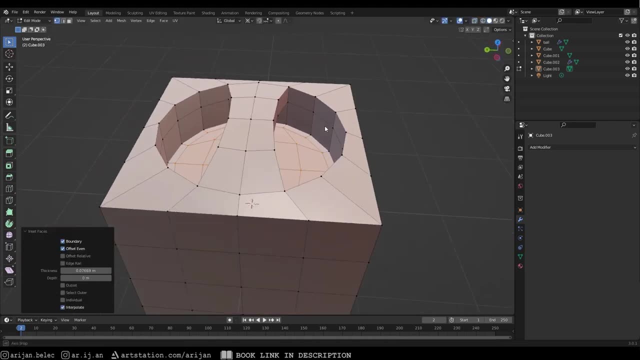 we're also going to select all these faces at the bottom and we're going to inset them a little bit here and we're going to add another edge loop over here, on the edge over here, just so when we use our subdivision surface modifier it's going to look a little bit nicer and tighter. maybe we. 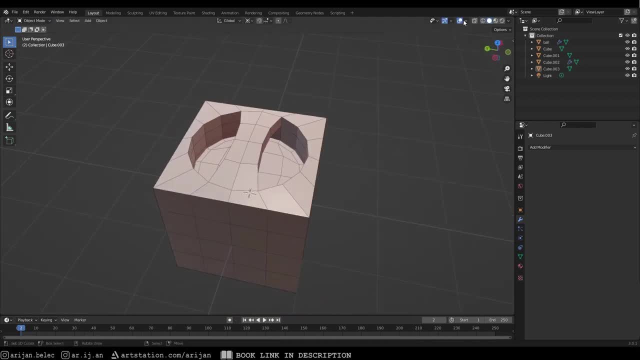 can add another edge loop over here on the side right. And now let's disable our wireframe view. okay, As you can see, now we have a bridge and now we just have to make it a little bit nicer using some subdivision surface modifier and some more bevels and stuff like that. okay, 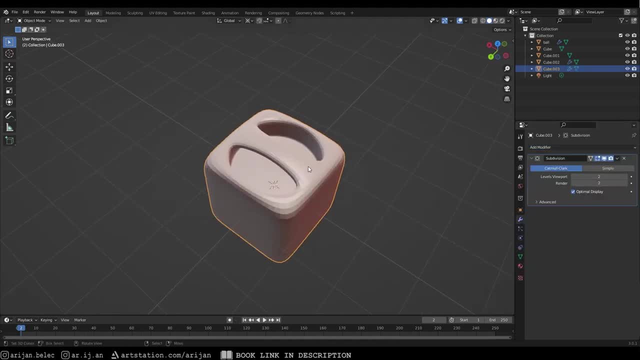 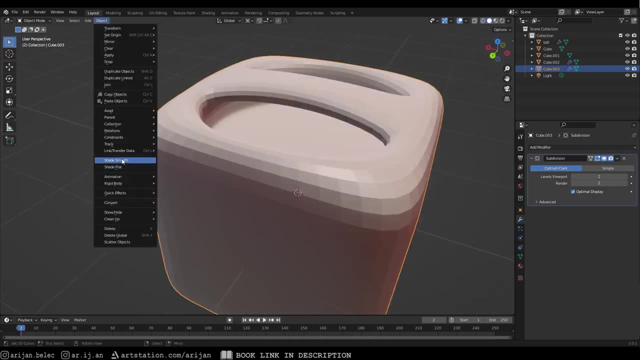 So we're going to add a subdivision surface modifier. as you can see, since we have perfect topology, this subdivides perfectly well, so we have no problems with that. no triangles, no angles. we're also going to add some smooth shading right here. okay, Now one detail that I want to add here. 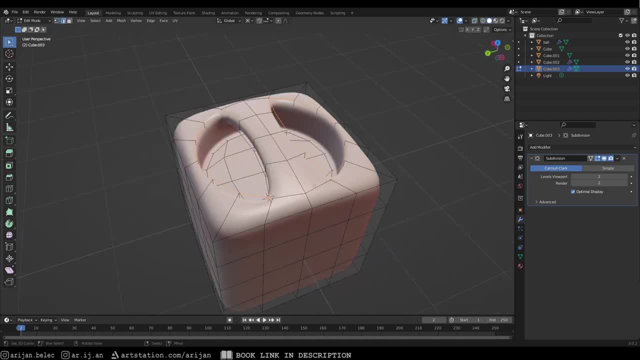 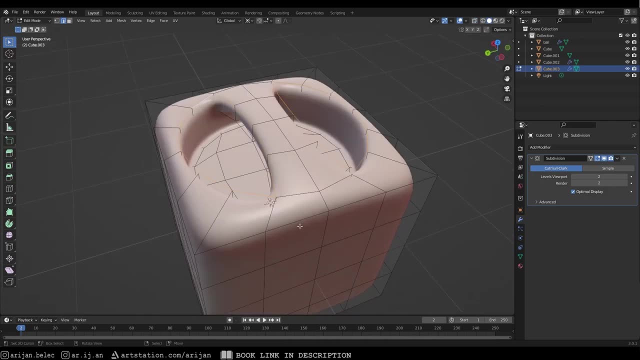 is, I want to select all these edge loops on the top here again around these two holes, so the sides of the bridge and the sides of the holes that go around by the bridge. okay, And once we have those two loops selected like this, we're going to press control B to bevel them a little. 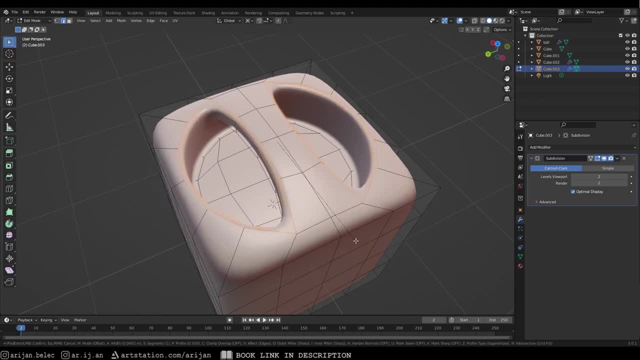 bit, all right, Something like this, just a little bit, Because that way, when we add some loop cuts to the sides of these bevels like this, it's going to look a lot nicer. all right, Check this out. 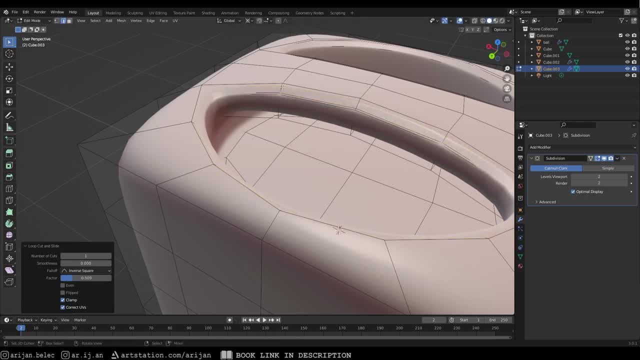 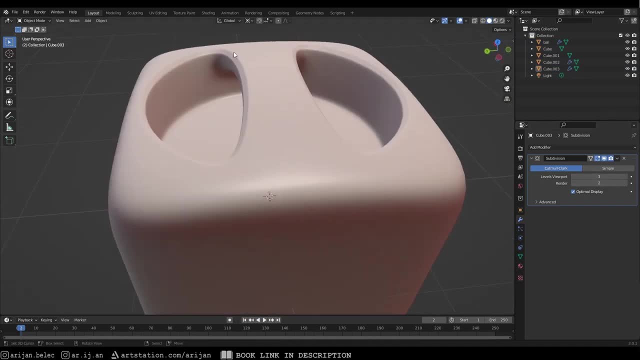 We're going to do the same thing on the other side, over here, and it looks a lot nicer because we have a nice bevel edge over here. We can add another level of subdivision and you can see that we have this nice, smooth, beveled edge over here. 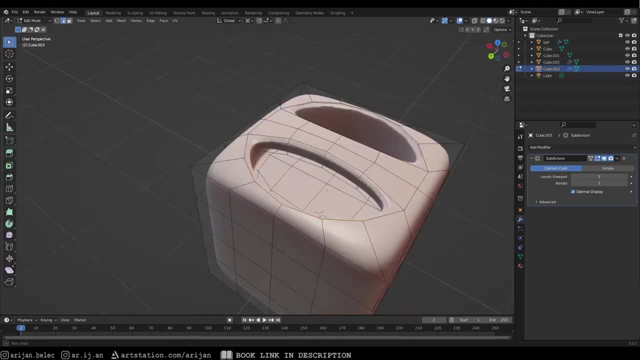 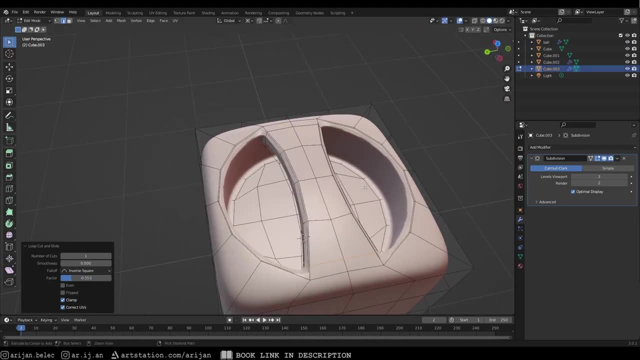 It looks much nicer. You can also add a couple more loop cuts. if you want a couple more loop cuts to the side here to tighten some of these edges. if you want to do that, I'm just going to leave it without those because I think it looks pretty good already. Maybe we 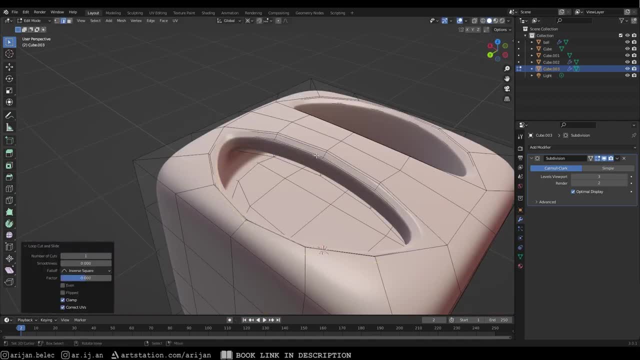 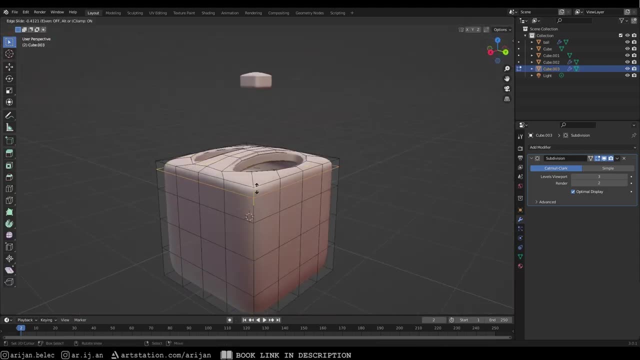 can add another two edge loops on the bottom here or loop cuts on the bottom here, so we can slide those down a little and tighten these edges a little bit. but we're going to leave it at that now. okay, Maybe also this side, because that's also going to look a little bit nicer. 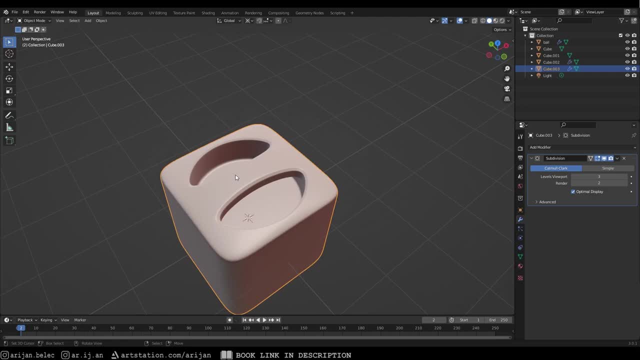 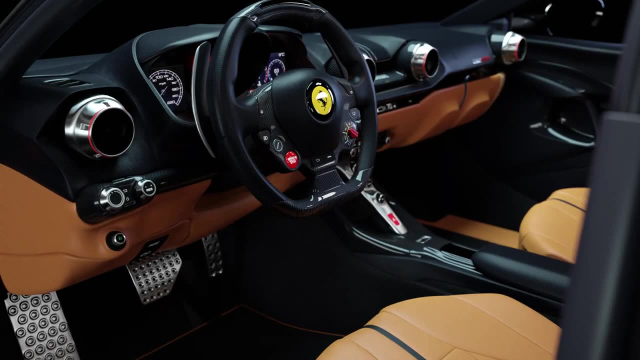 As you can see, now we have this perfect bridge connecting the two sides of this hole, so think about what kind of situations you might be able to use this for. For example, I made a Ferrari once and there were a couple of parts where I needed to have a handle, like this: going over a gap and 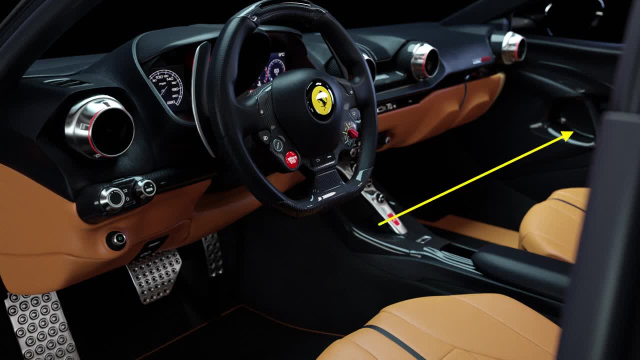 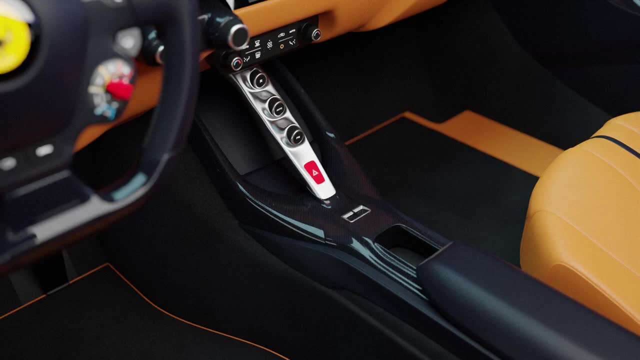 connecting the two opposite sides, For example the inside car handle or the door handle on the inside. it needs to be a similar shape like this. There's another shape in the central console of that particular car which required me to do something similar, so this can be useful in a lot. 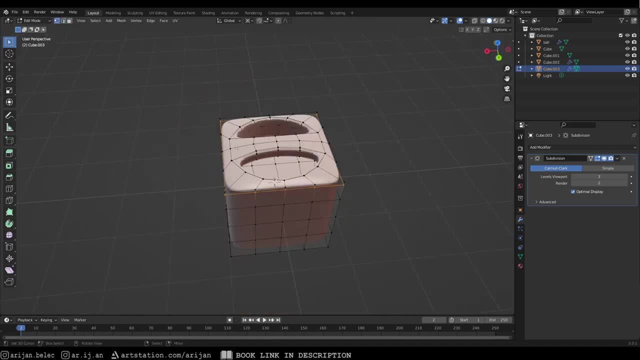 of cases, but in any case, exercising your topology is probably one of the best ways to improve your modeling skill. So if you guys enjoyed this, click, like and subscribe, and I hope to see you guys in the next one.